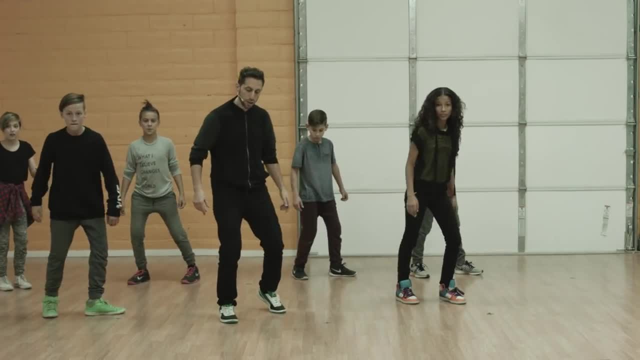 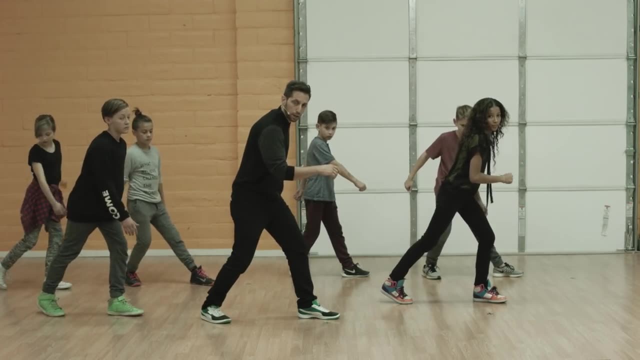 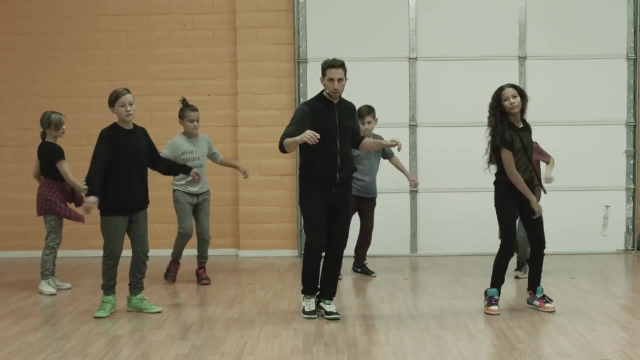 behind you. two, step three. Then you're going to kick with your right step back on your right step behind the left kneecap step and spin. OK, I know that was a lot of movement, so we're just going to review that for you. OK, so from here, your last jump. 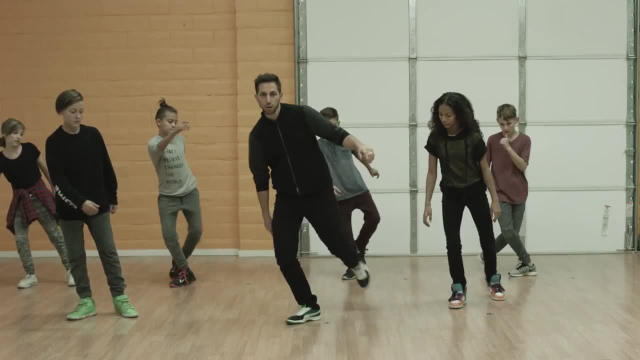 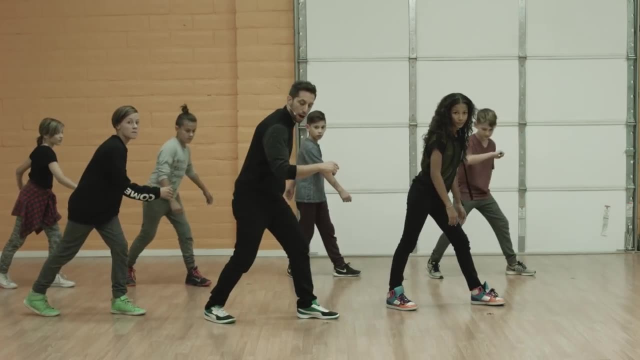 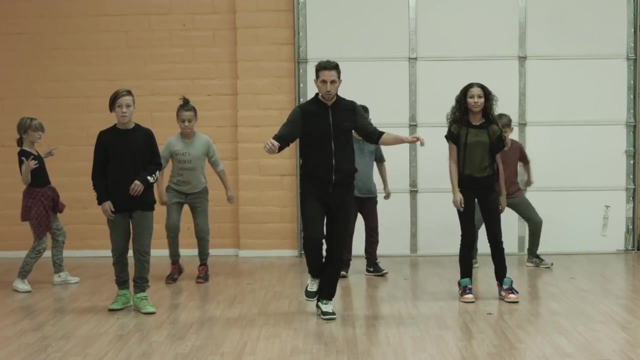 You've got one behind the right foot, two and three. The kick happens with the right foot. on four, You step back five Behind the left knee. six, Step back again seven. Then you're going to turn to your left shoulder. eight, OK, moving on from there Right out. 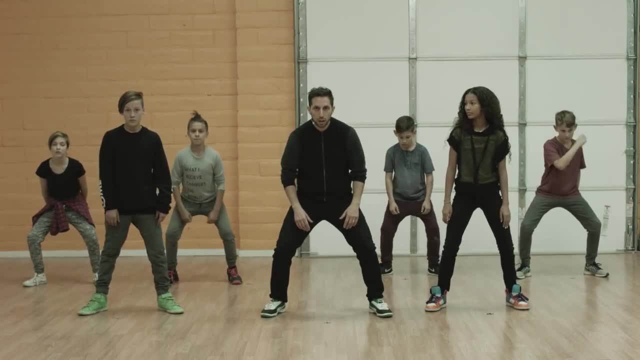 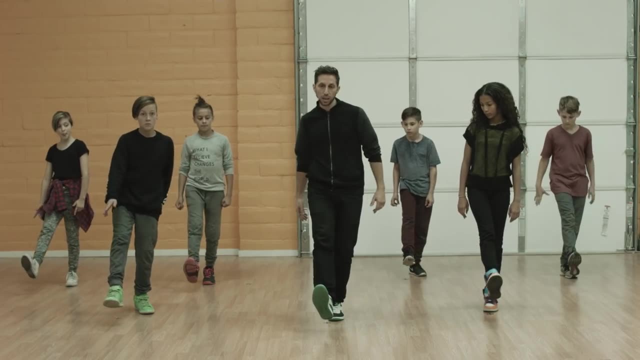 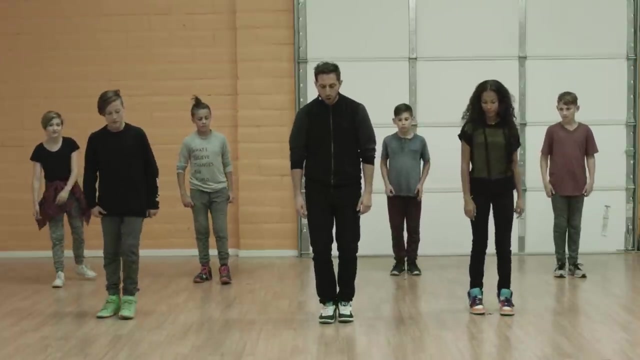 of that turn. you're going to plant your feet one, Then you're going to bring them back in. two Right foot's going to kick, Kick as you go back. Kick, switch left, switch right. OK, let's do that. 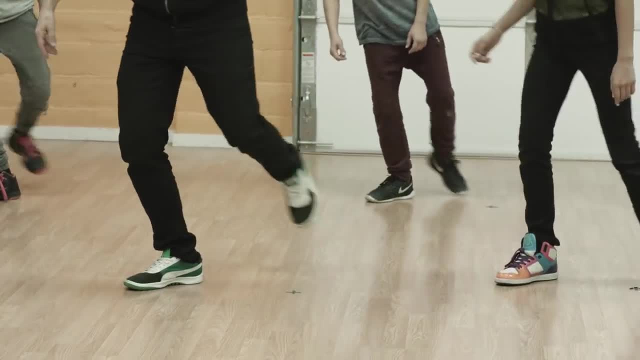 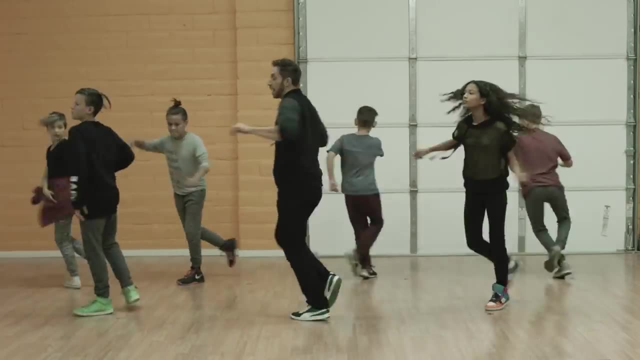 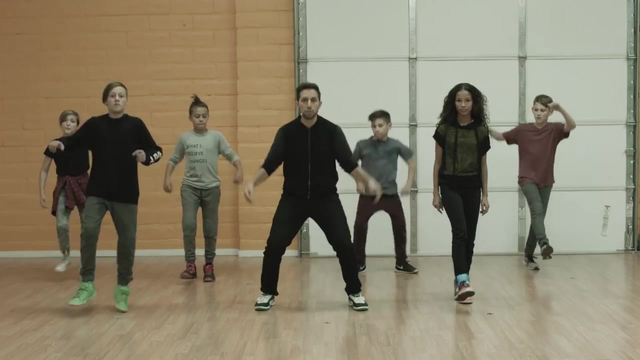 So we have from the step out, guys, we're going one, two and three, Kick four, five, six, seven, Spin eight. one, two Back, three and four From here, drop five, Pull back. 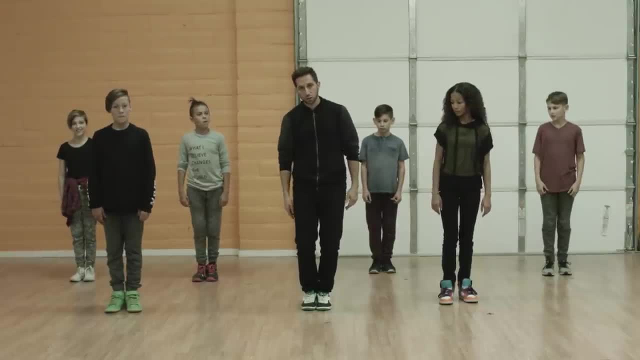 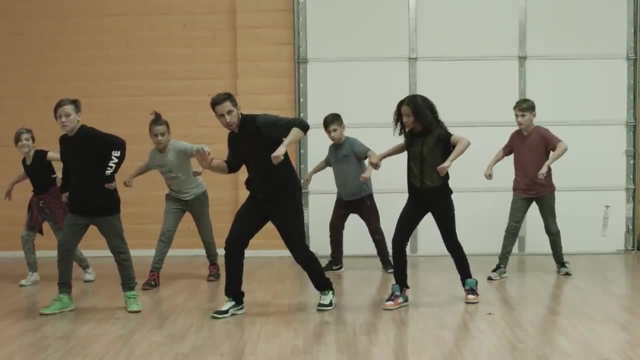 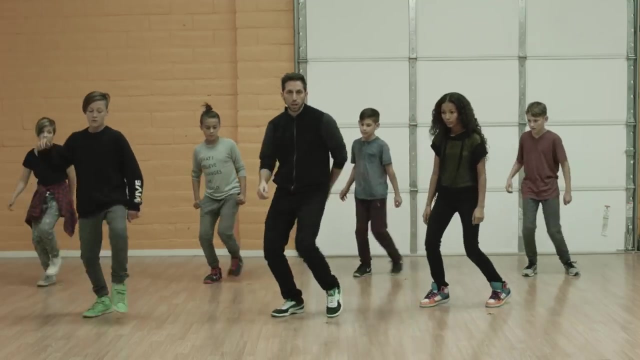 together: Six, Then you're going to step on a diagonal to your right. seven, So you bring these elbows up here. seven and you hold for a single count of eight. OK, let's take it from the top. Here we go. You've got right foot one, two, three jump. 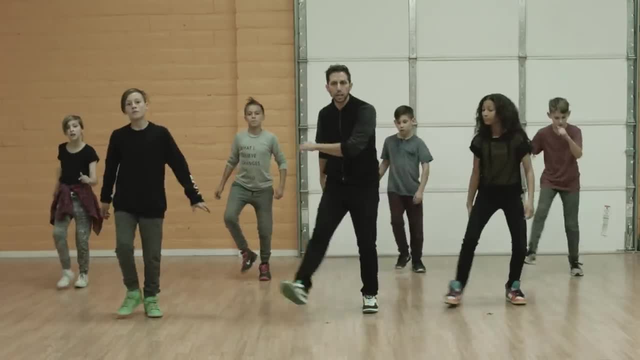 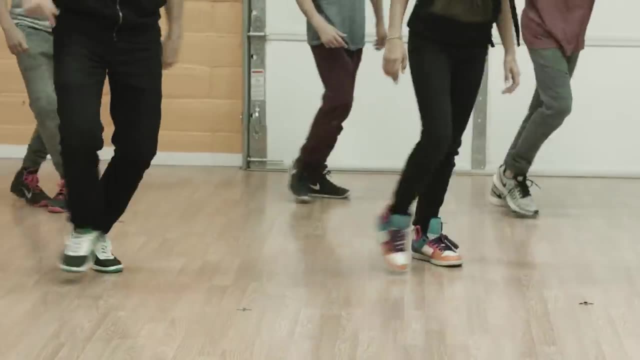 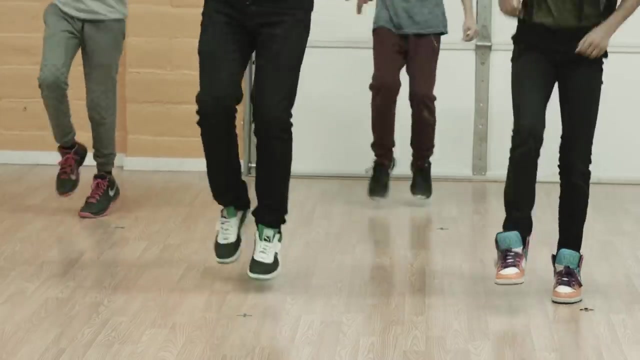 four Left, five, Right, seven, eight, Again one, two, three jump and left right, left jump One, two and three, four, five, six, seven, eight, One, two back, switch back drop. 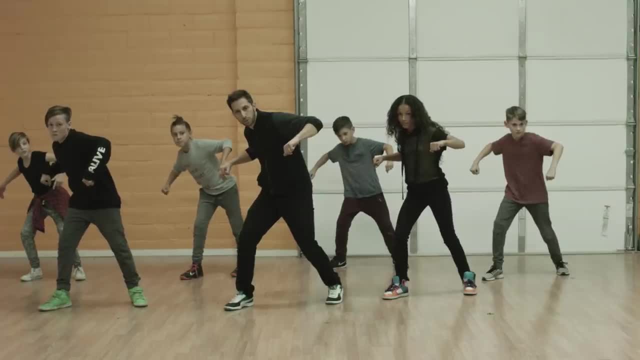 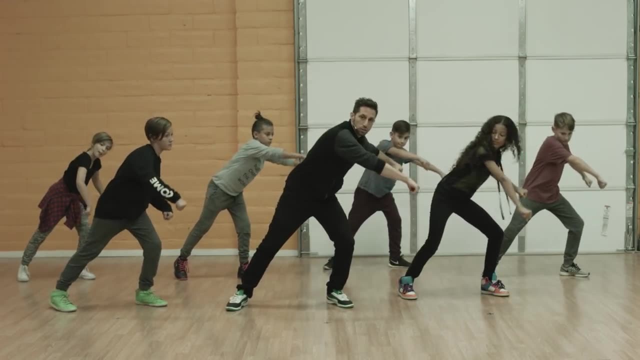 together. hold Moving on from here. You hold for that single count of eight, Then you go to your left shoulder, stepping out with your left, and you're going down in a semicircle going one, two. Good OK. 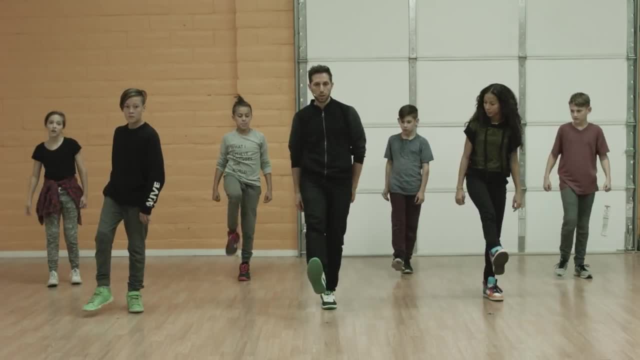 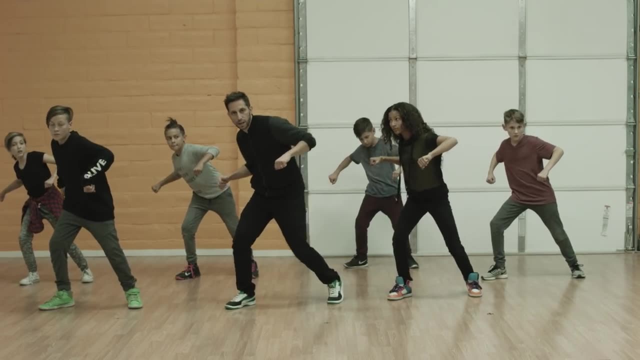 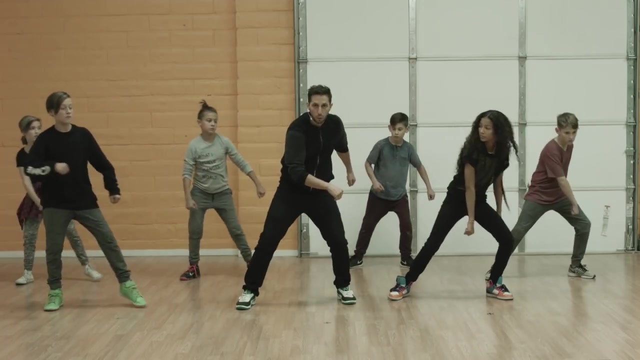 Let's go back From here. kick switch back goes five, six, seven, hold eight, Then one. two step back with your left. three, Then bring it back. four, Then you're going to do a leg. 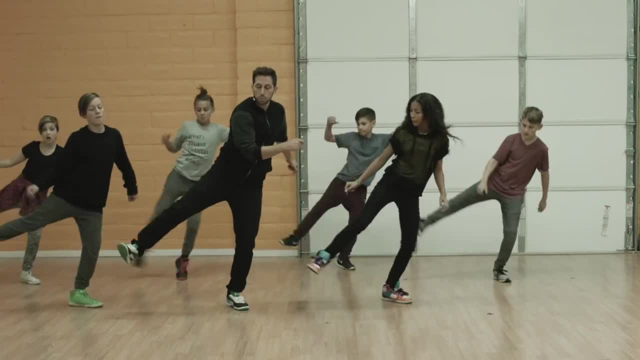 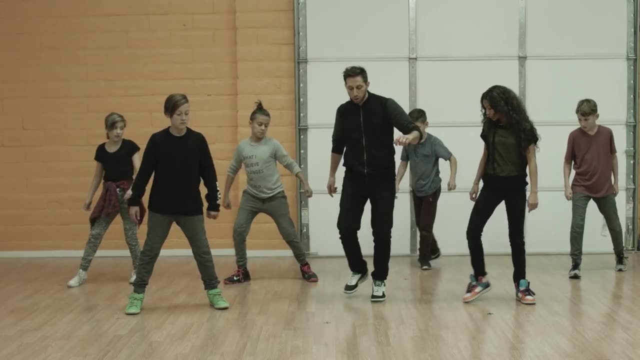 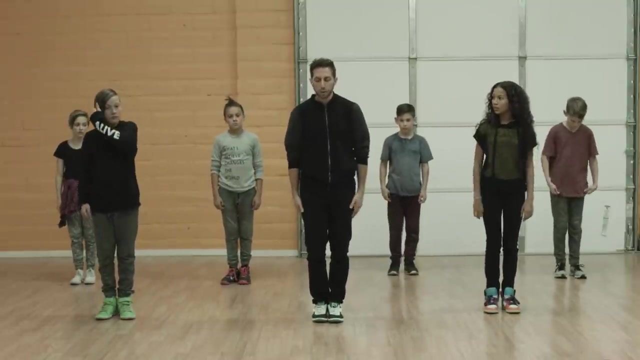 sweep, So your left leg is going to kick the right leg out. Sweep, step over in front. Left leg comes behind. Here's a little tricky footwork: Right goes behind step. OK, Let's do that again. So from here, let's take it, guys, from this movement right here. 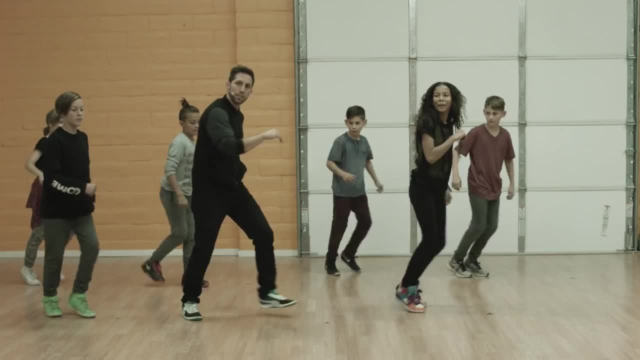 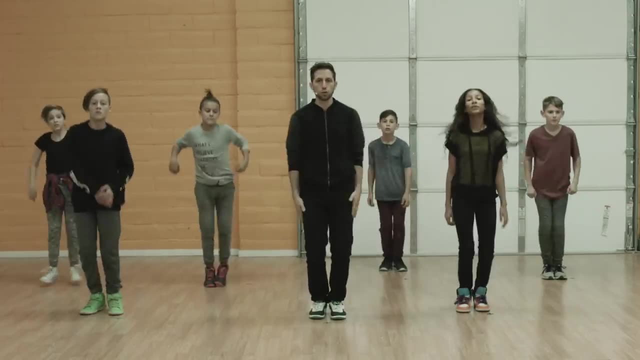 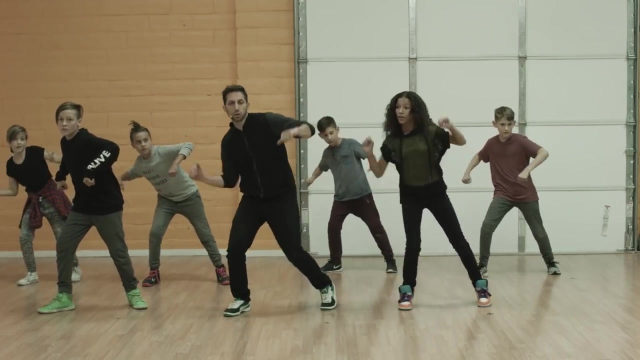 OK, We've got one, two and three. kick four, five, six, seven, spin eight. one, two right, three and four. drop five together. six hit seven. hold eight, circle one. 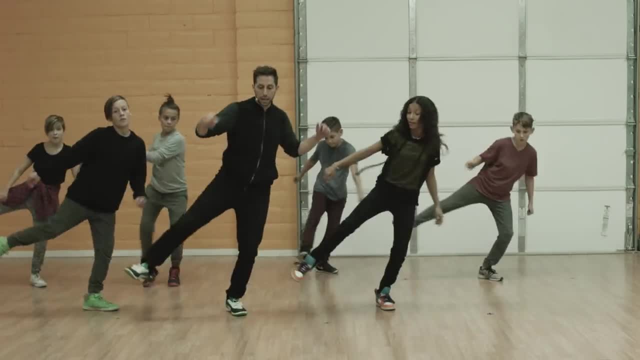 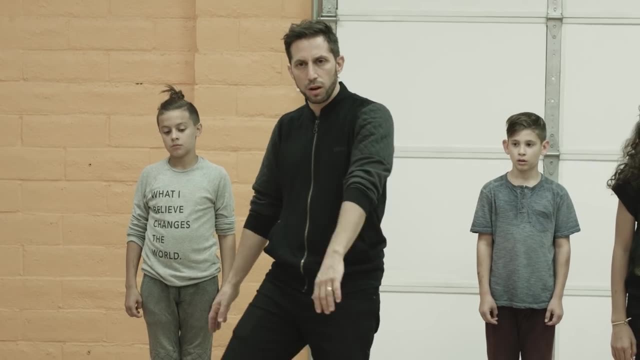 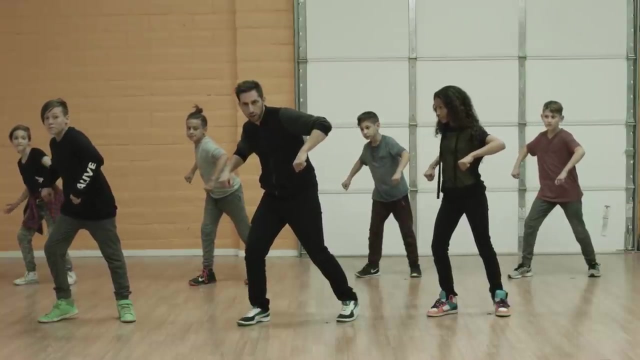 two Step behind Together, Sweep the leg. six, then seven and eight. OK, So I want to go over that eight count where we last left off. We were here on seven and we held for the single last count, which was eight. Then we step with our left arms, go. 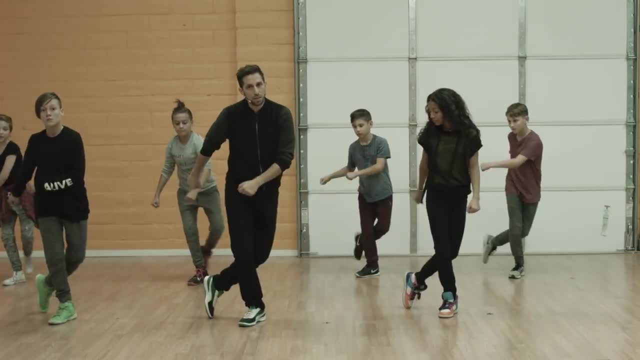 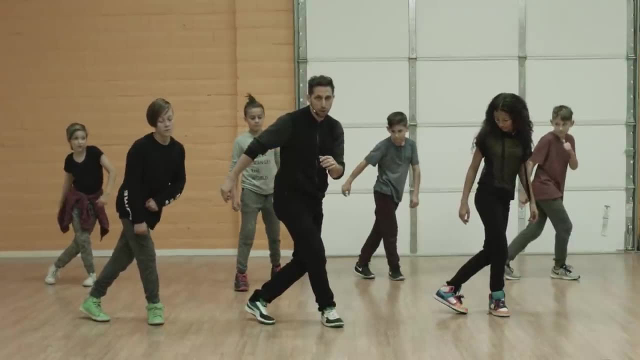 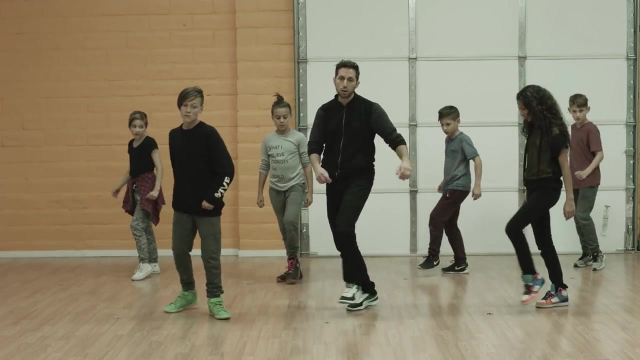 across. We're going one, two step behind three, come back out. four. Now you leg sweep five, step over six. Now from here You're going left foot's, going to step seven. then you pull your right back, end and cross. 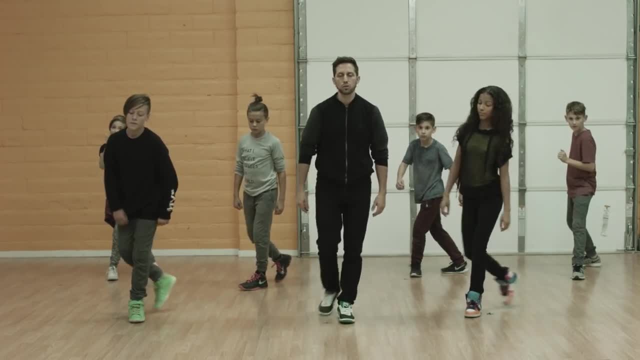 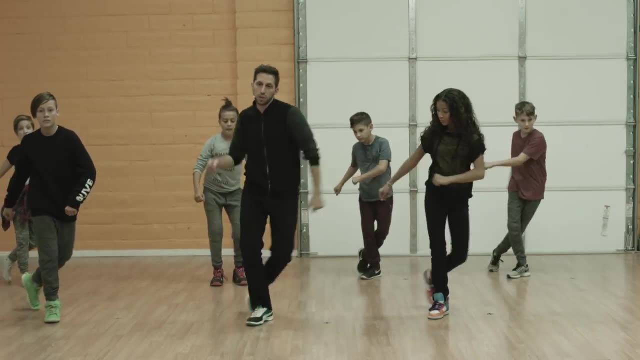 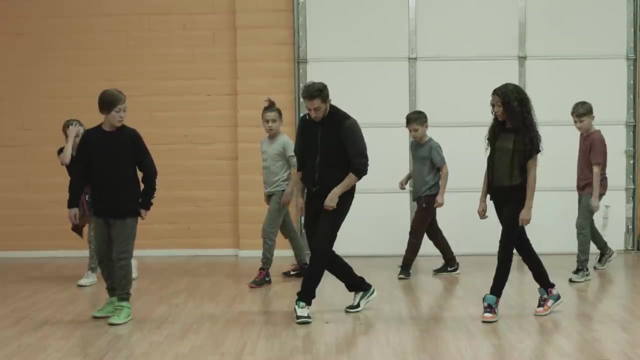 over eight. OK, All right. So let's try just that. from here, Seven hold eight goes one, two, three, four, five, six, seven and eight. Good Moving on. So from here we're going to connect our right toe to our left ankle. 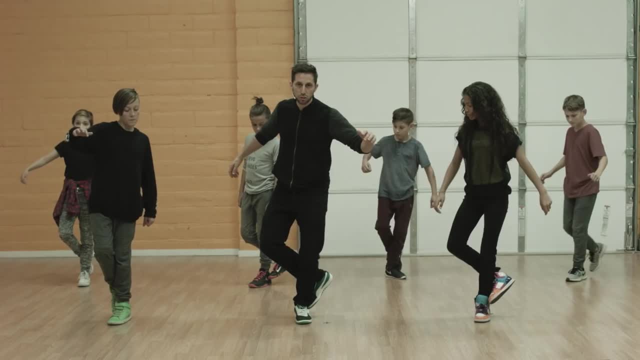 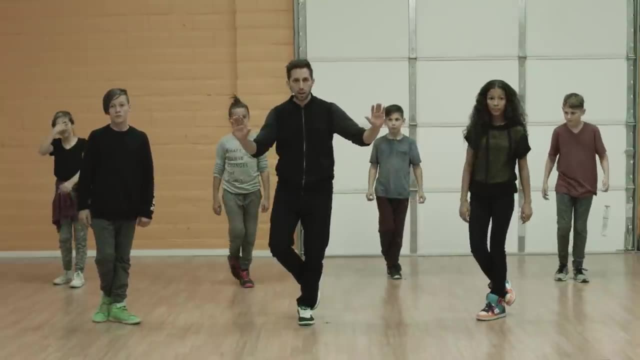 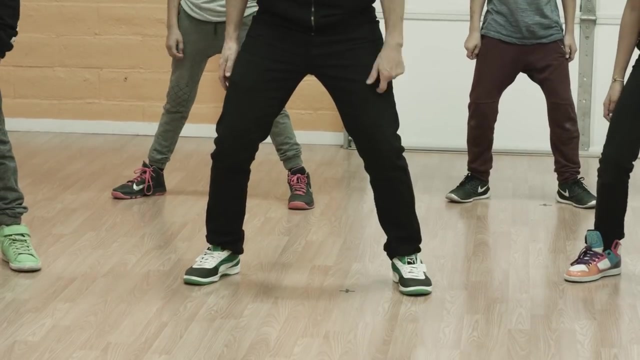 OK. So what you're going to do after you make that connection, you're going to turn four times: Turn two, three, hold From there. this right foot is going to kick out, kick in out. Then the left goes kick. so I pulled my right there in out. 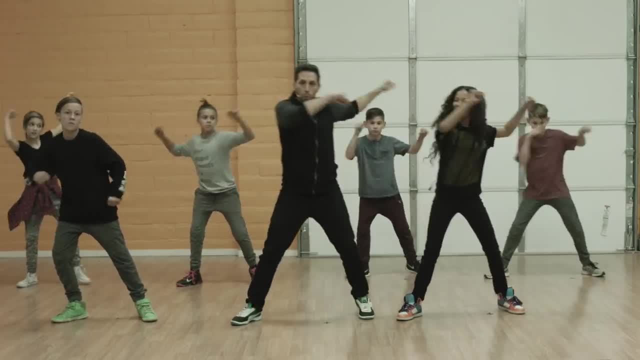 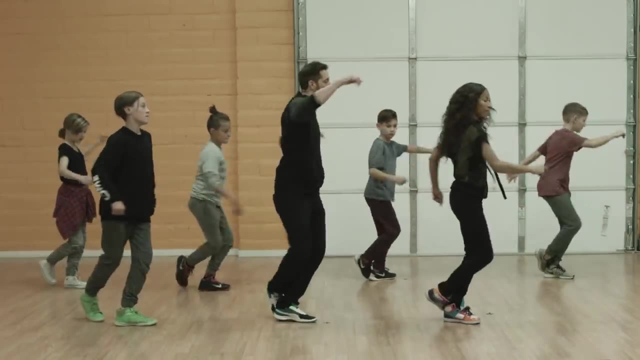 Good, Let's do that. one again Goes. one, two, three, four Sweep five, Six, seven and eight. Then it's turn two, three, four, kick in out, kick in out. 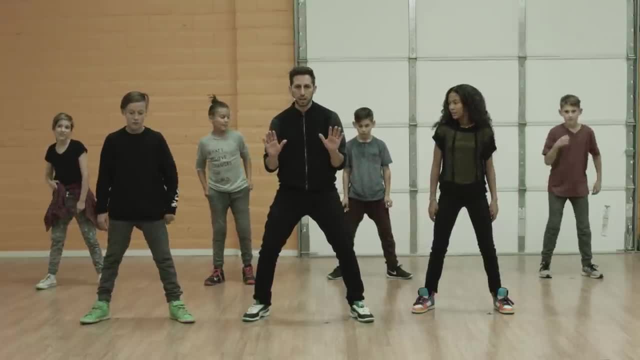 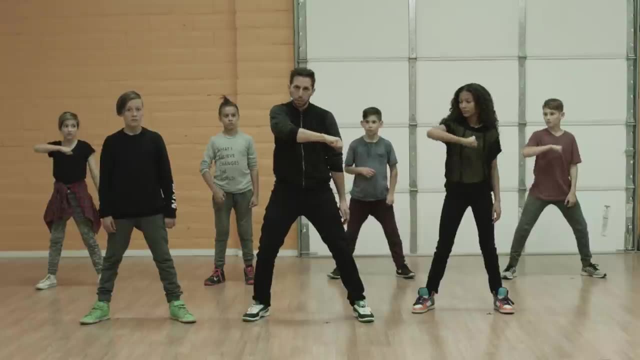 Good, All right, We're coming up on the last eight count of the dance, and so what we're going to do is we're going to go right fist across the body and we're going to go one, two, three, four. 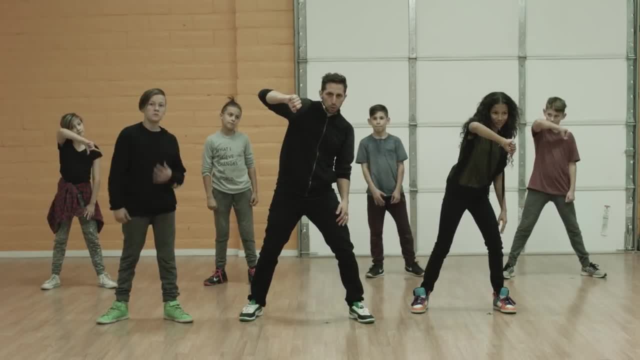 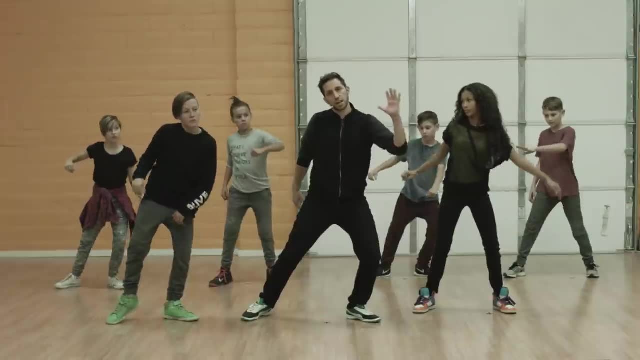 OK, Kind of like you're looking out of a window pulling a curtain back. All right, One, two, three, four. Then we switch to the other side quickly with the left hand and go opposite way. five, six, seven, eight. 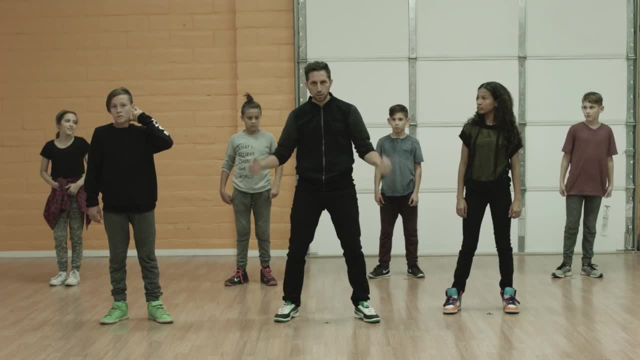 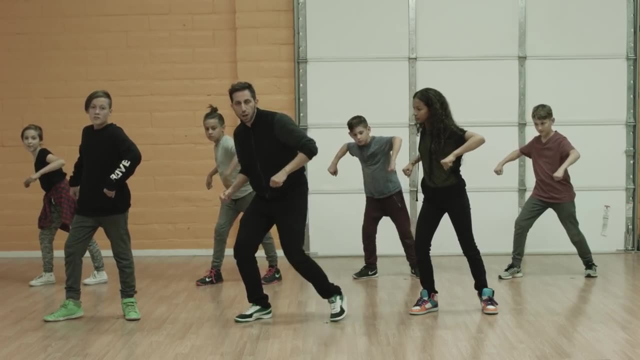 So notice that we went lower each time. we did it OK, All right, So let's take us back to here and then we'll walk it through from the top Seven holding eight going one, two, three, four. 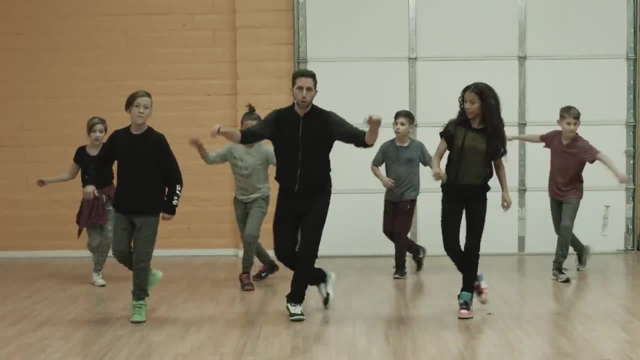 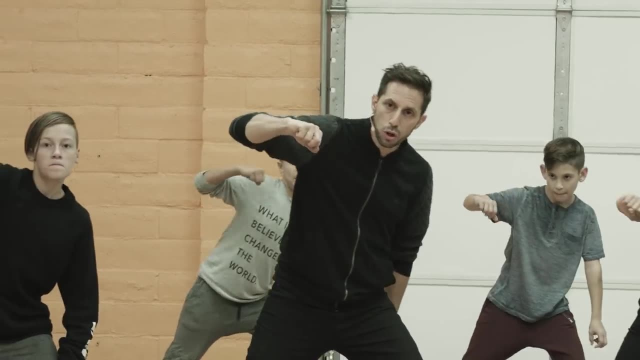 Sweep, five, six, seven and eight, Turning one, two, three, four, Kick five and six, seven and eight. Then it's one, two, three, four, Then five, six, seven, eight. 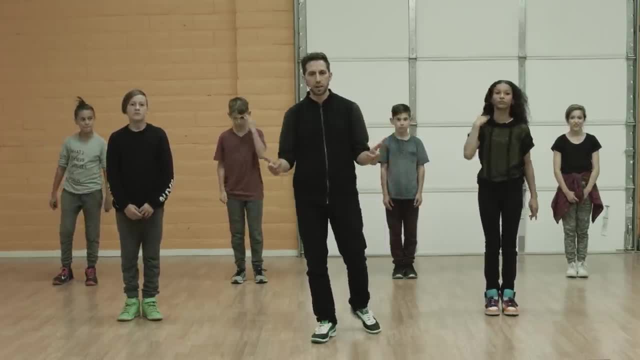 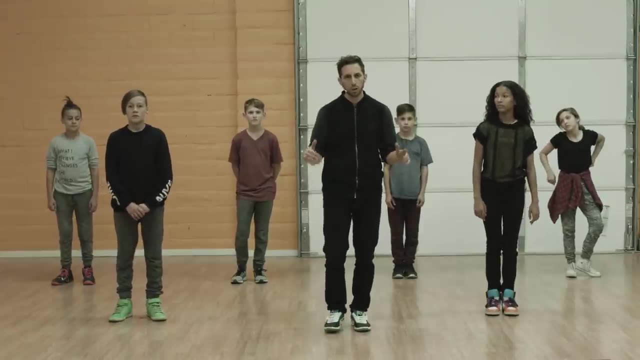 OK. So now that we've walked through the breakdown of verse one, we're going to take it from the very top, without stopping. We're going to go at a medium pace, just walking the whole dance through, Ready, Starting with the right foot on. five, six, seven goes. 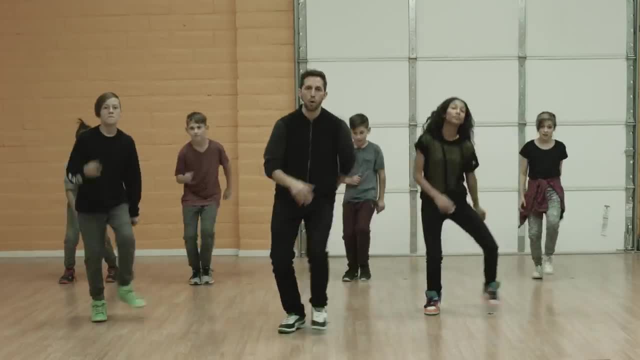 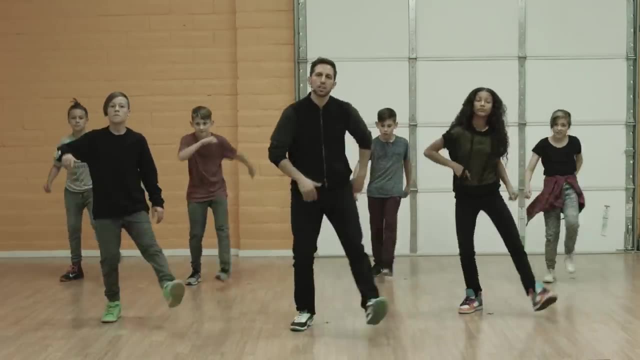 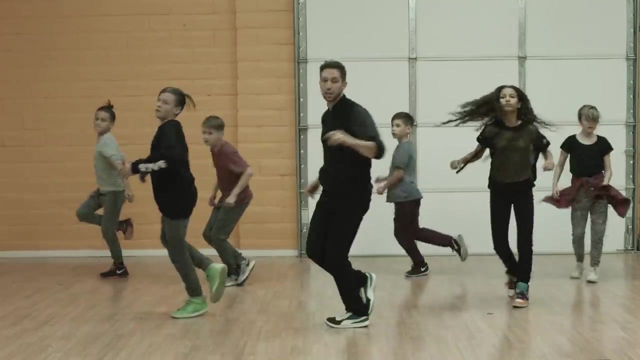 One, two, three, four. One, two, three, four, five, six, seven, eight. One, two, three, four, five, six, seven, eight. This is one, two and three. Kick four, five, six, seven, turn eight, one, two, back three and four, five in. 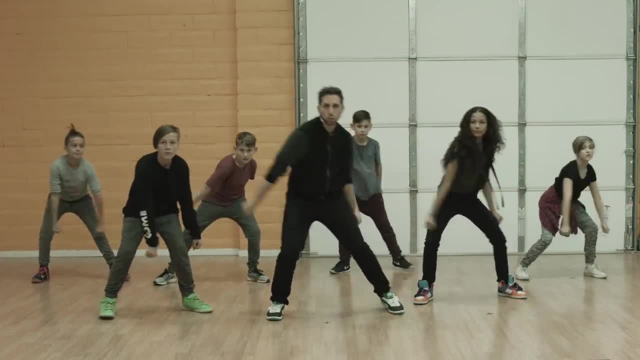 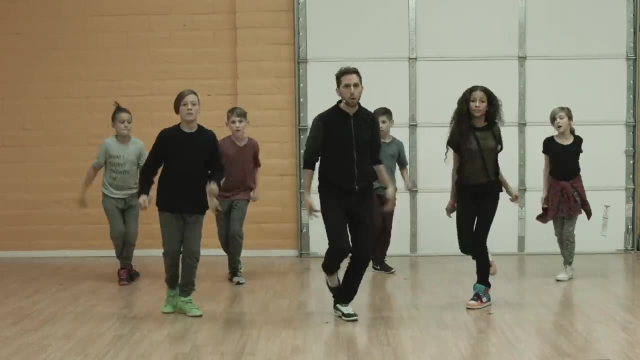 six out seven hold eight. Then it's one, two, three, four, Sweep the leg, cross, tap, tap, tap. Then one, two, three, four, Kick in out, kick in out. 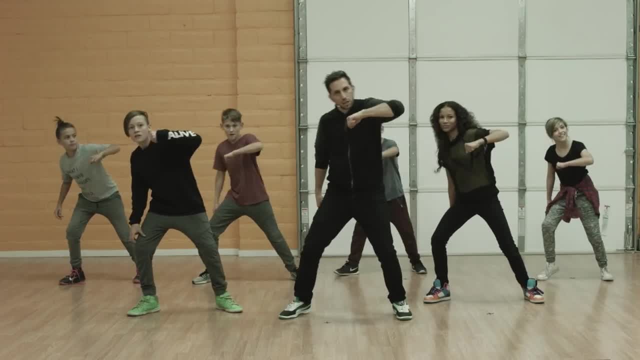 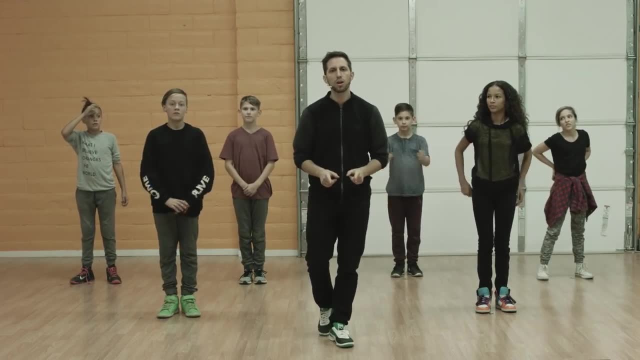 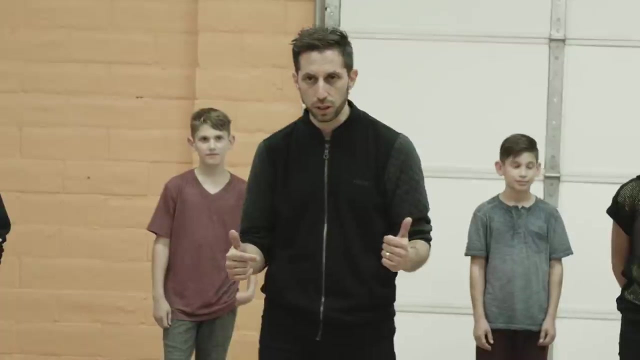 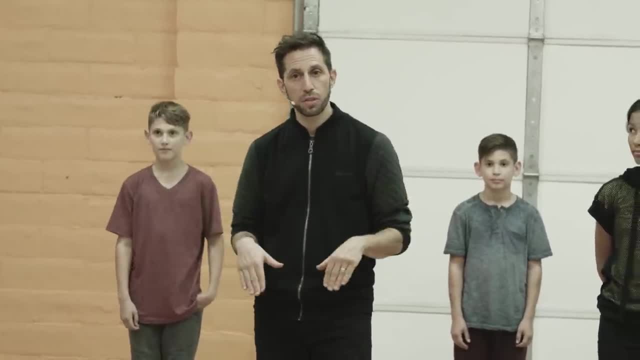 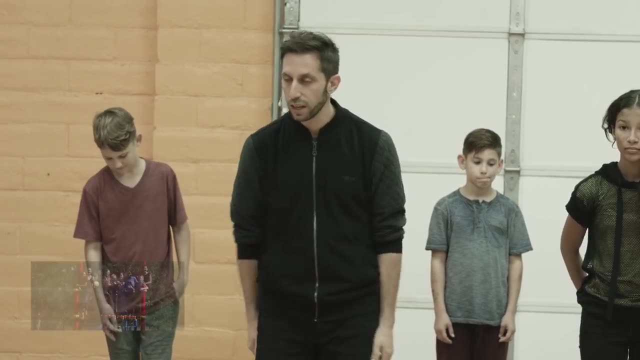 Now I want to warn you: it is fast, So try and keep it up with us. If you need to, you can always rewind, Rewind, Review the material and then try it again at the tempo. OK, Here we go with music. 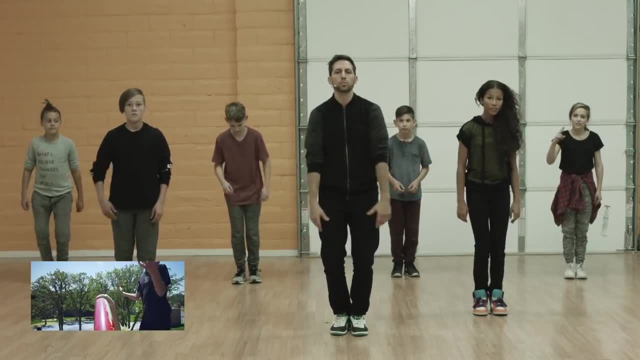 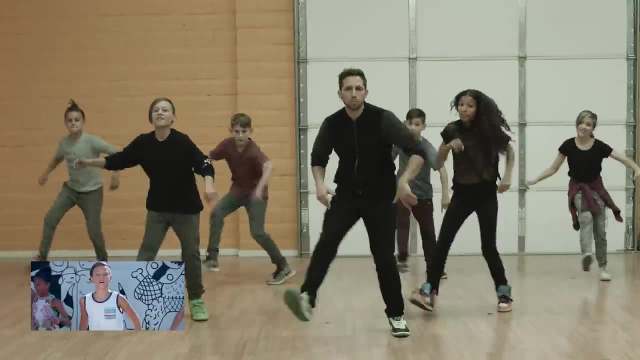 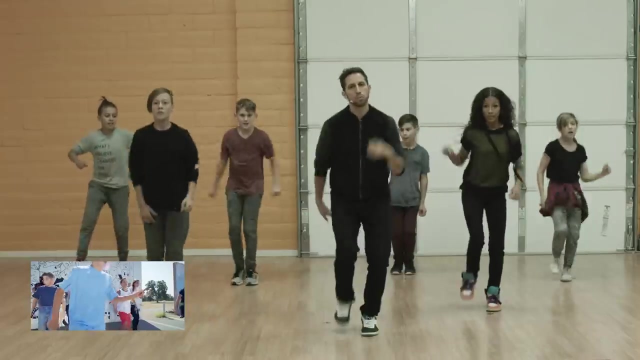 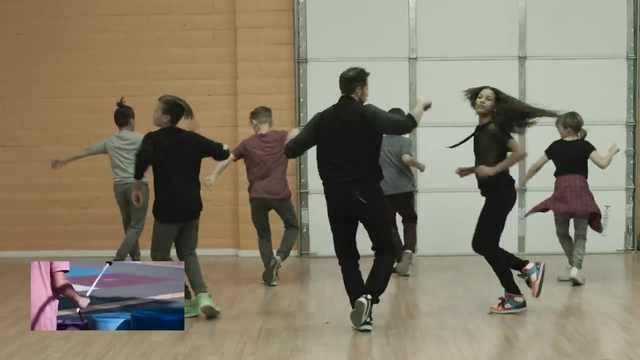 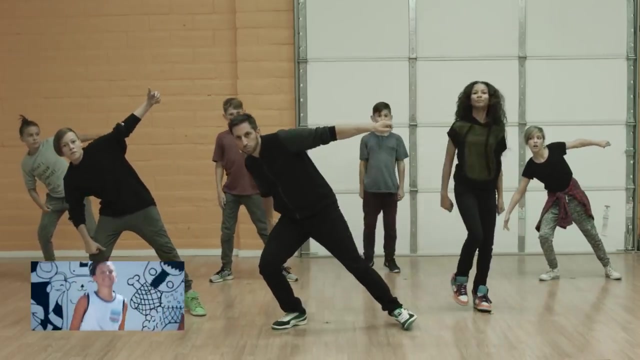 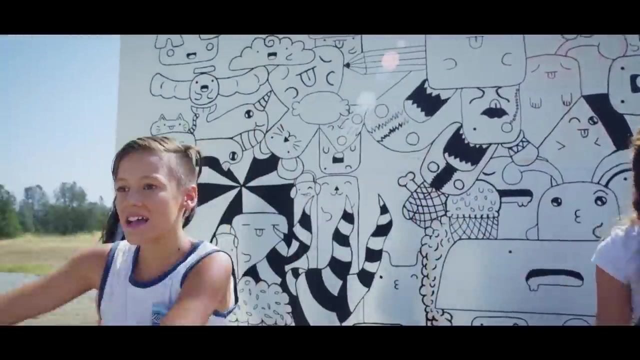 Five, six, seven, eight, Ok, Your kindness fills my life, Your love amazes me And I sing because you are good And I dance because you are good. 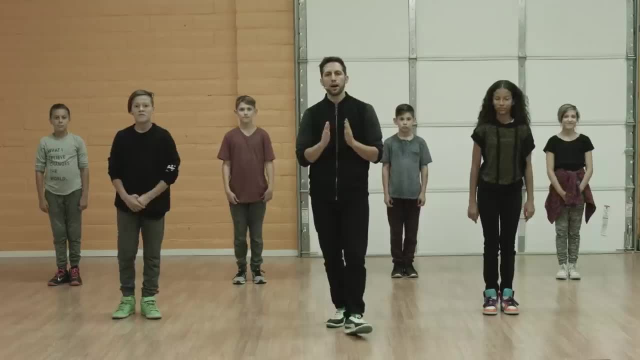 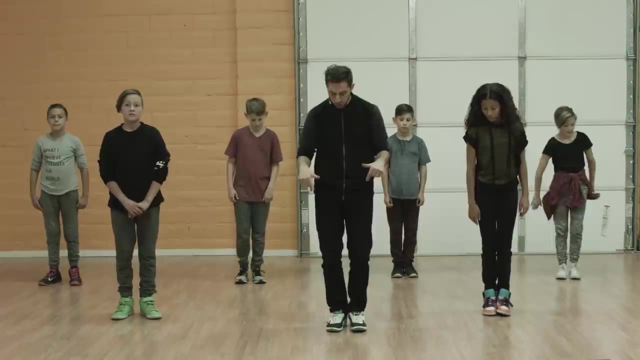 And I shout because you are good At this point. now we're going to move into the chorus of You Are Good, So we're going to start first. Everything works well with the lyrics of the song, So I'm going to start first, though, with the feet. 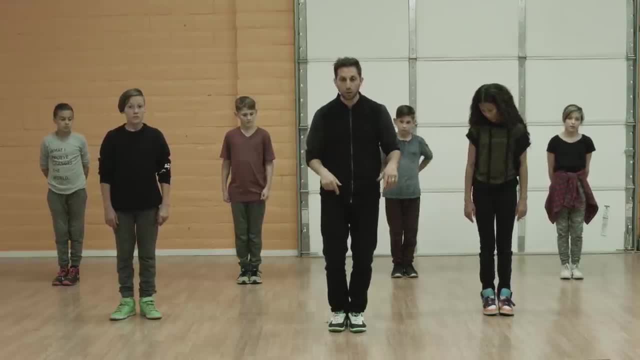 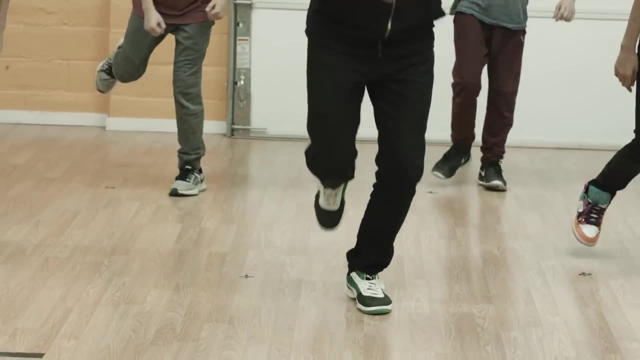 and we're going to add the arms later for the first eight count. So the feet are going to go onto the right foot for two counts. Hop hop, Then onto the left foot, Hop, hop. Then you do singles: Right left, right left. 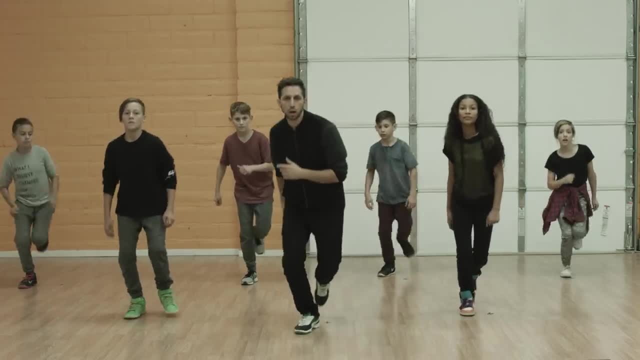 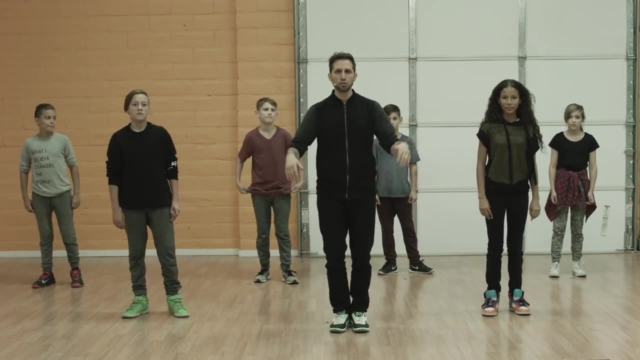 Okay, So our footwork for the first eight count is 1,, 2,, 3,, 4,, 5,, 6,, 7, 8.. Okay, Now just the arms. You're going to punch the right arm up. 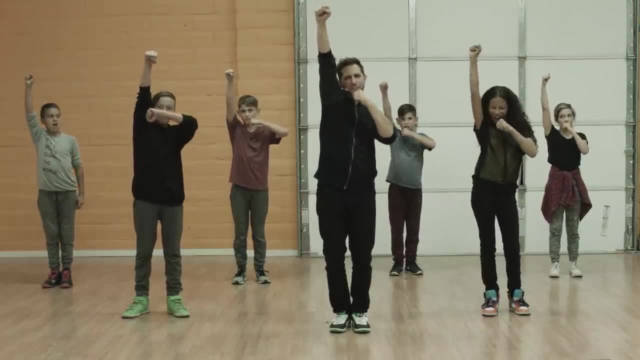 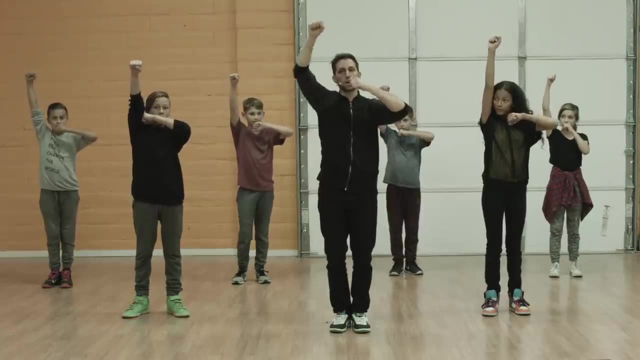 left arm out like a rock star, like singing on stage right. So you've got 1, 2.. You're going to hold this position for 3, 4.. Then you're going to switch four times: Switch, switch, switch, switch. 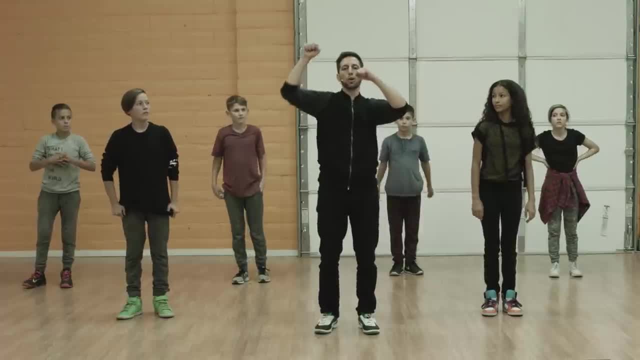 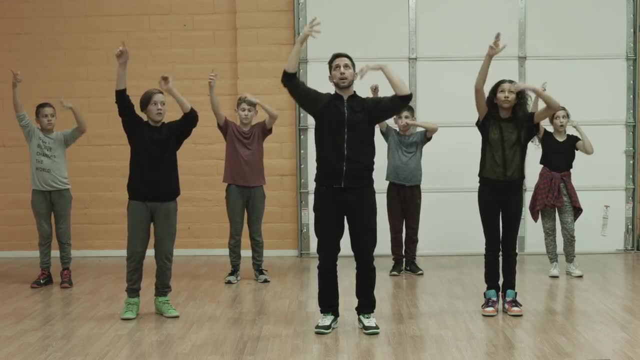 Okay, So lyrically it happens that you go and I sing because, And then on the UR you'll actually open up the hands and direct it upwards that you are good. Okay, So putting them together, arms and legs, slow. 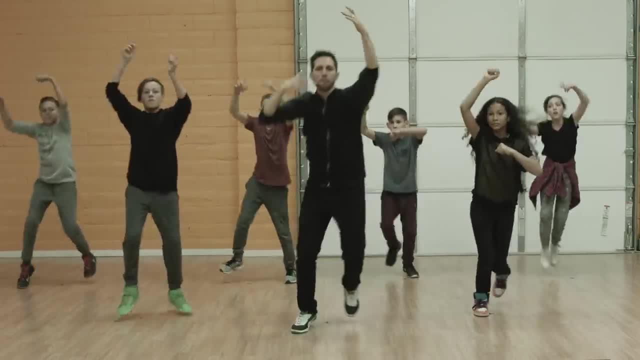 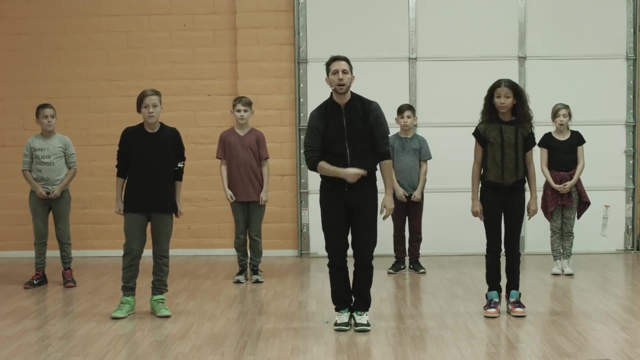 we're going to go 1,, 2,, 3,, 4,, 5,, 6,, 7,, 8.. Okay, That's our first eight count. Let's repeat that: 5,, 6,, 7.. 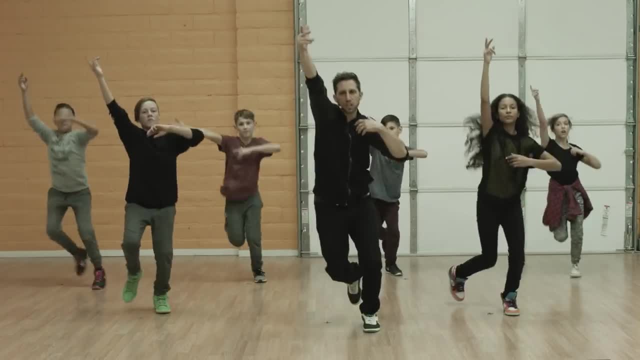 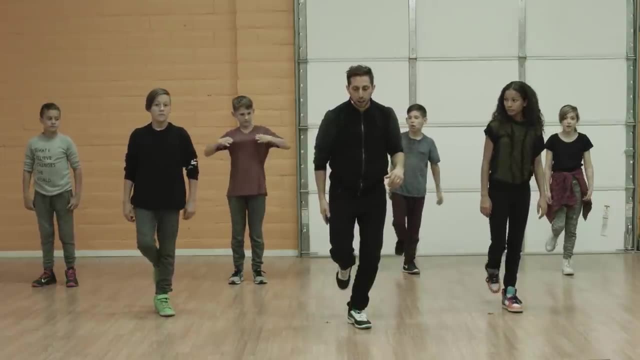 Goes 1,, 2,, 3,, 4,, 5,, 6,, 7, 8.. Good, Now, moving on from here, notice that your right foot is up in the back. You're going to take that right foot forward and slide. 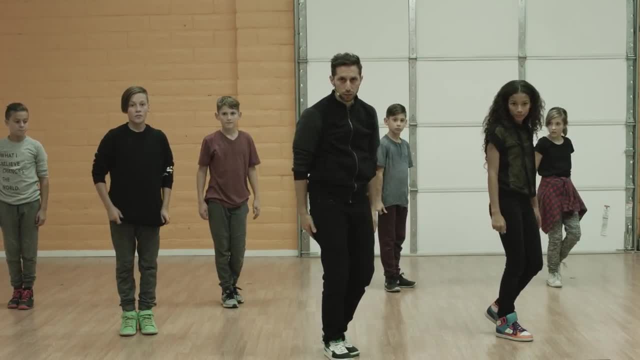 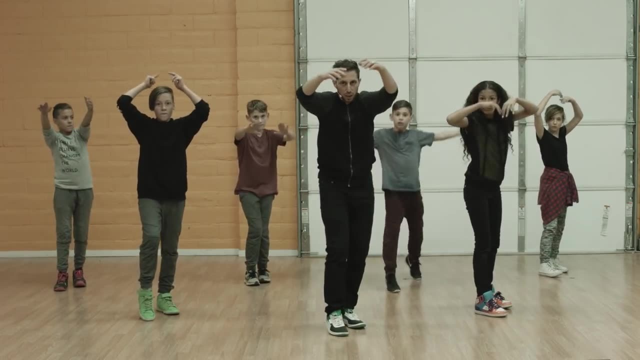 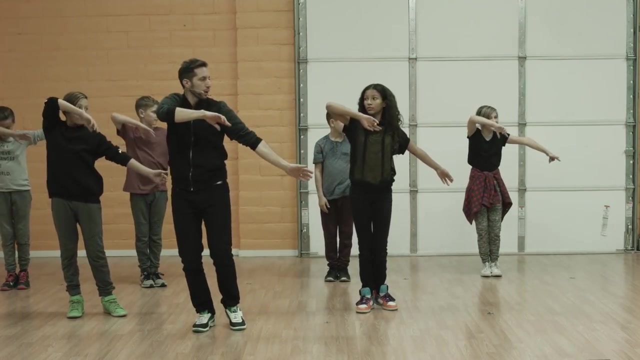 Arms open and come down, Then you're going to slide back. That left foot is going to lead the movement now and the arms come in reverse inside, Then you're going to slide to your right, sliding over arms over your head, and then sliding to your left, arms over. 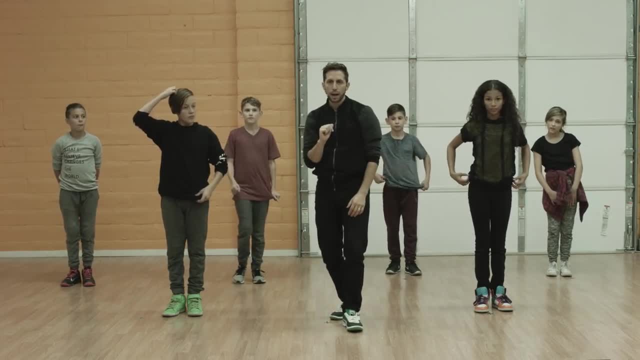 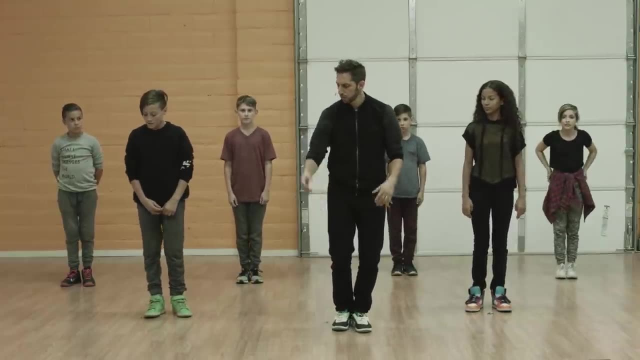 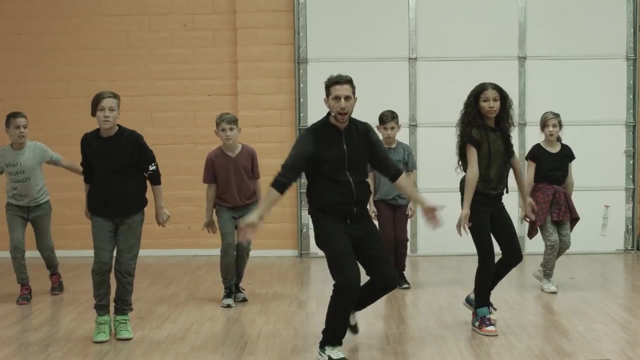 Okay. So if you know what I'm talking about, notice, we went forward and back and then right to left. Okay, So you're going to go from here. Give me from here guys, just from that next part. So sliding forward 1, 2, back 3, 4, then 5, 6,, 7, 8.. 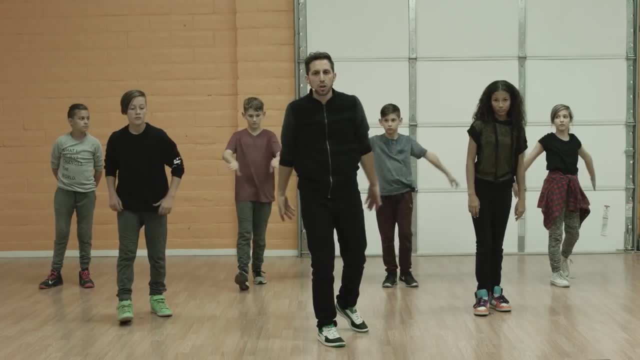 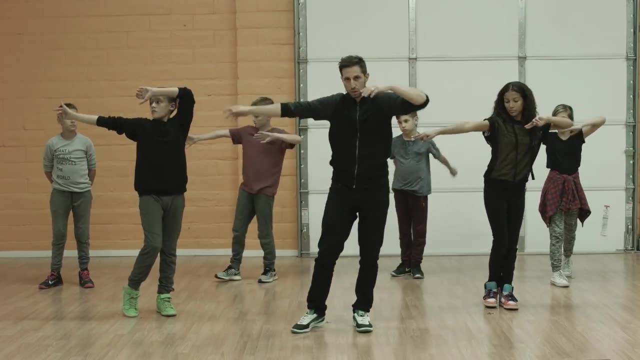 Okay, And the arms are that They open, then they close and come in and then they travel over The head and stay at the shoulders and then over the opposite way. Okay, Let's take that from the top Ready. 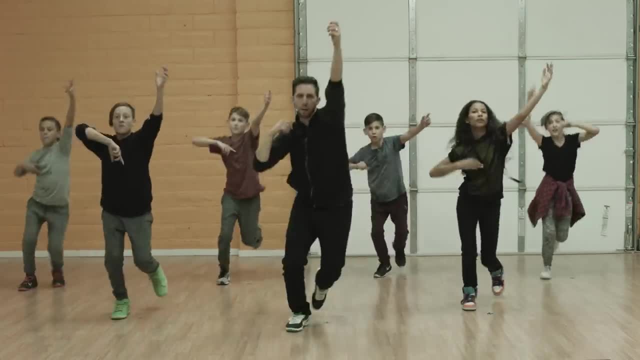 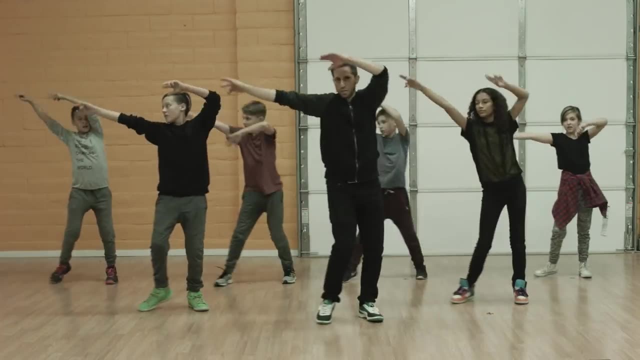 Goes: 1,, 2,, 3,, 4,, 5,, 6,, 7, 8.. 1,, 2,, 3,, 4,, 5,, 6,, 7, 8.. Good. 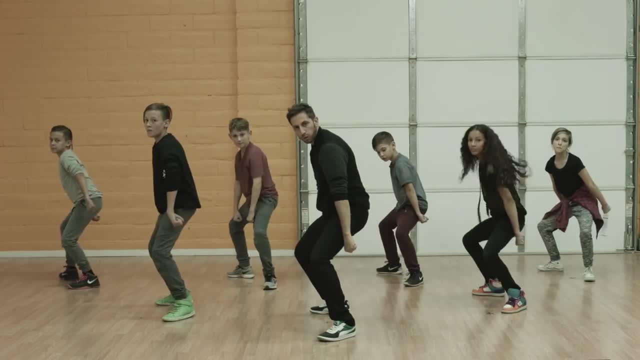 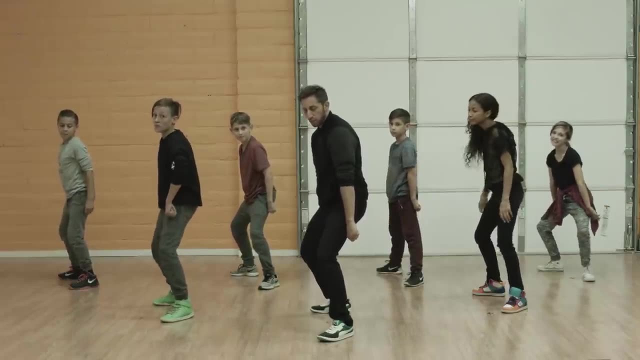 Next part You're going to drop Boom. Good, When we get to the lyrics, you'll understand what some of these movements connect with From here. then your arms come up, Boom. So you have some options with the hands. 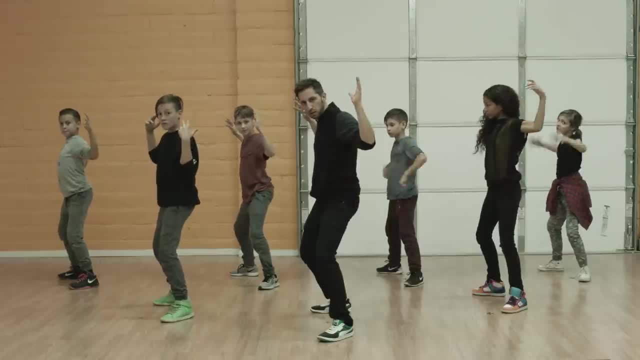 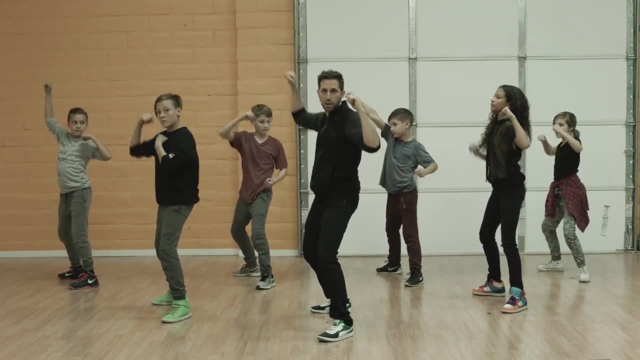 Either you can keep them in fists or you can bring them open and out, like this. But on this next part, your fists are going to pump 1,, 2,, 3,, 4.. And as they do, your left foot stays planted. 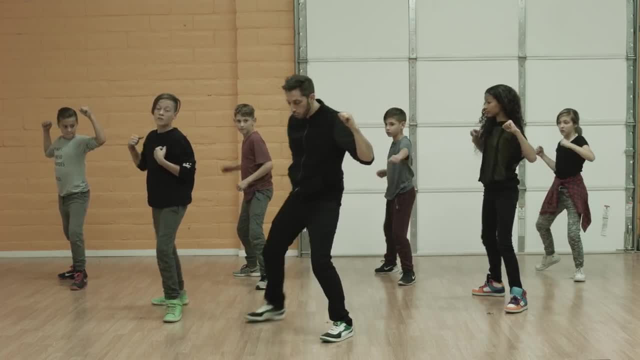 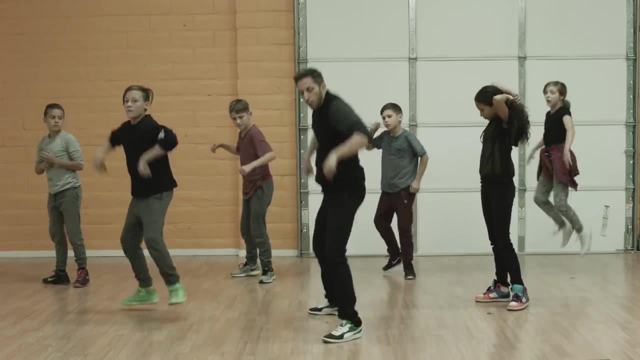 and you're going to pivot with this left foot, pick up the right and go 1,, 2,, 3,, 4.. Okay, So, putting it together from the drop, boom, boom. Then you're going to go: punch, punch, punch, punch. 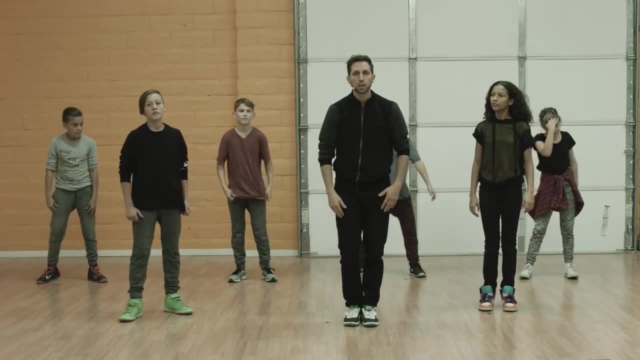 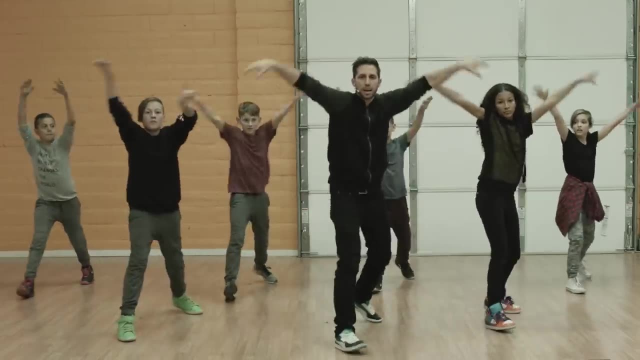 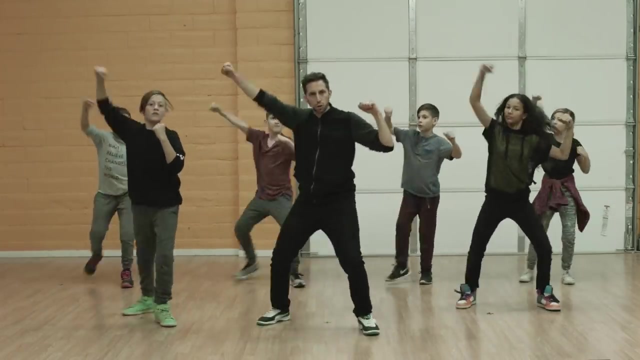 Good, All right. So, lyrically, from the top, you're going to be going sing because you are good And I dance because you are good And I shout because you are good. Okay, All right. So here we go. 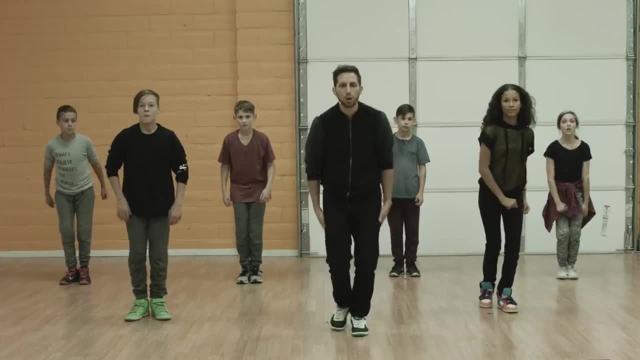 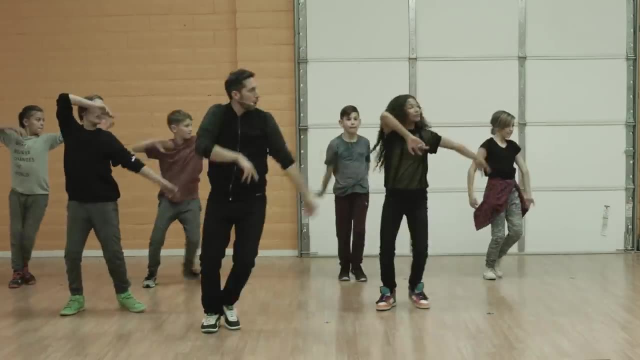 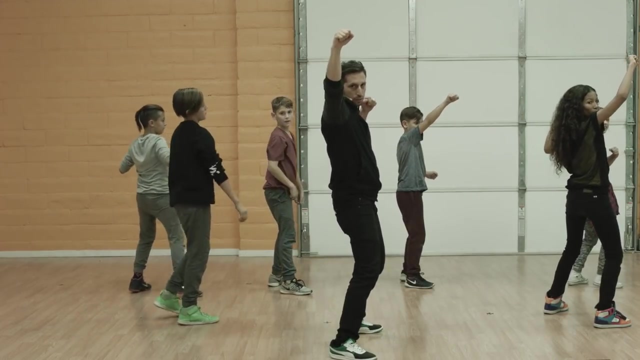 From the top of that, 5,, 6, ready. go Sing because you are good And I dance because you are good And I shout because you are good, Good, All right. And on this next part, right here, 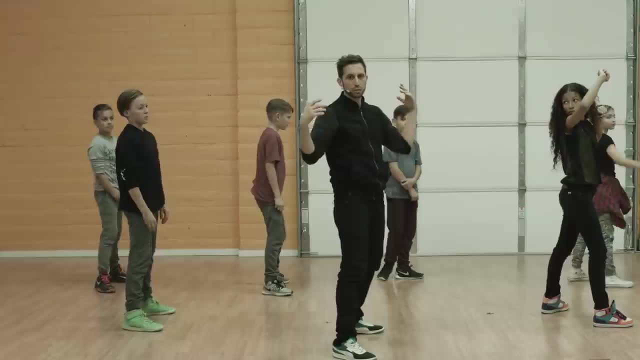 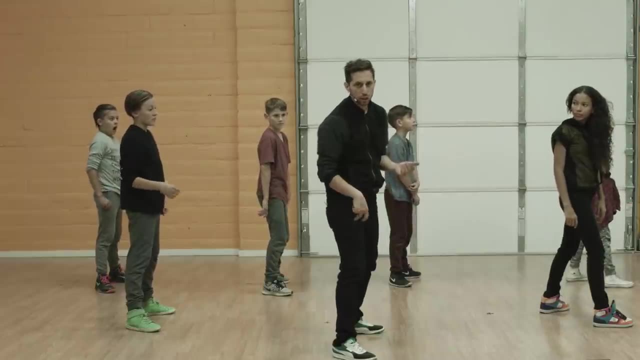 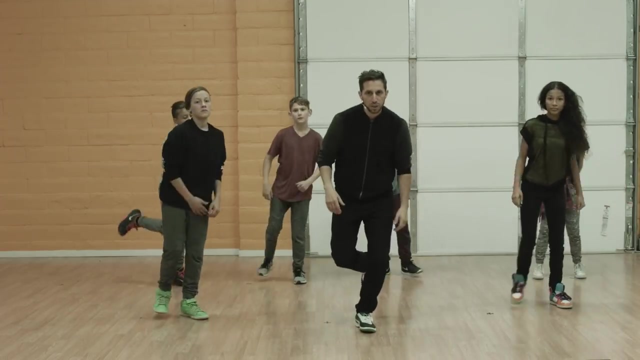 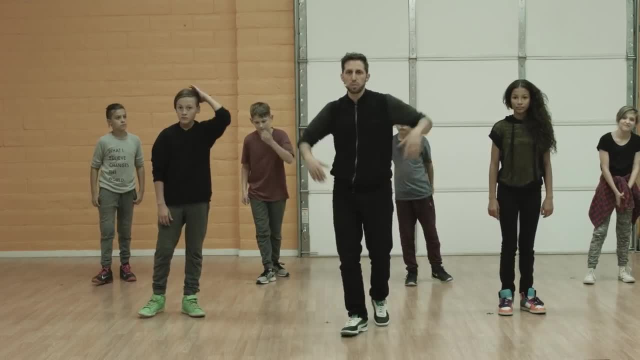 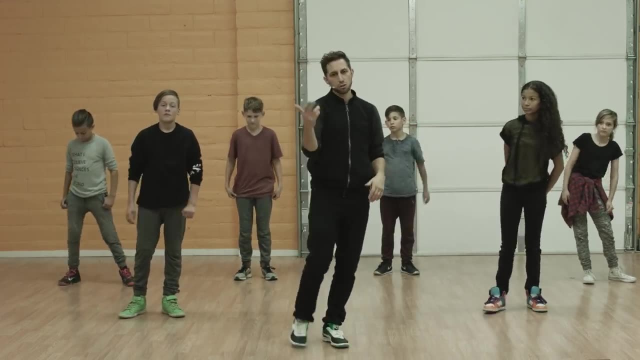 So that's the basic footwork, but you're going to put yourself into it. It's basically just like a dance of freedom. You're just kind of celebrating the last aspect of the truth that's in this chorus. Okay, So here we go. 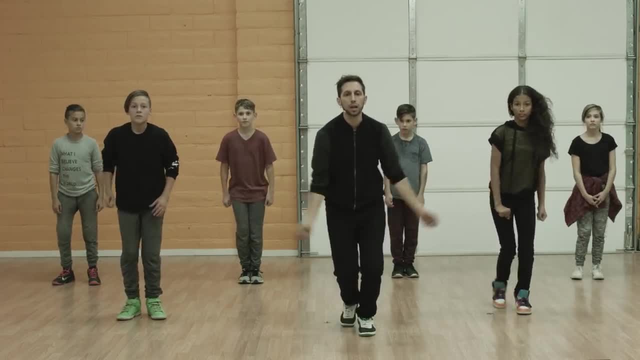 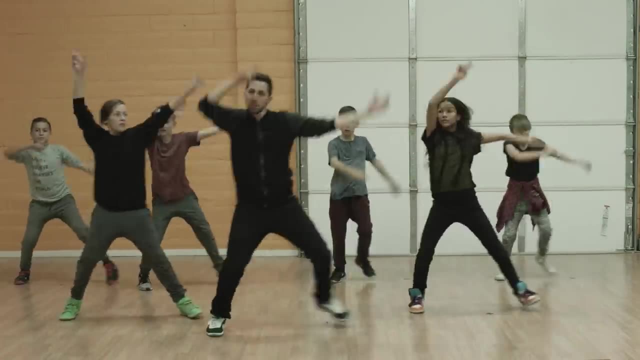 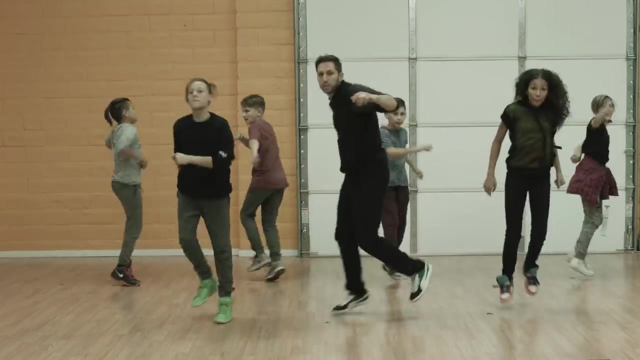 Let's walk it through from the top Ready and sing because, Because you are good, and I dance because you are good and I shout because you are good, you are good to me. Boom, Okay, You can get as expressive with the arms as you want. 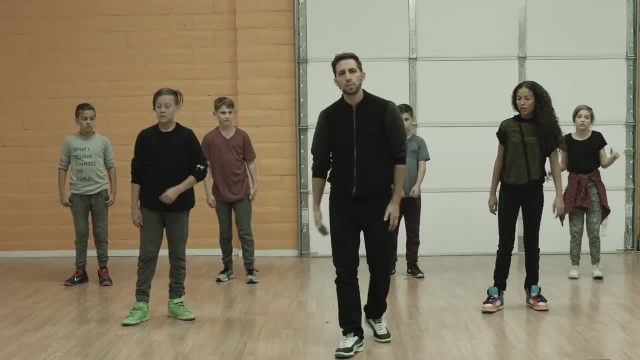 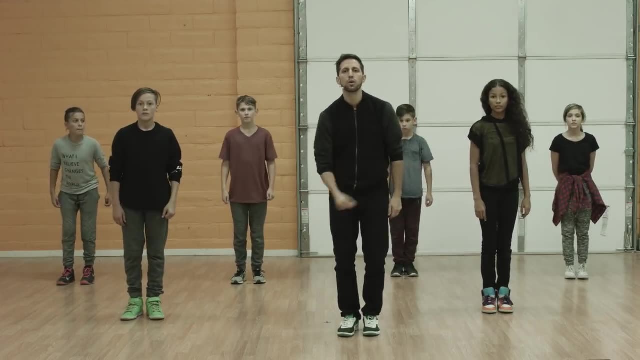 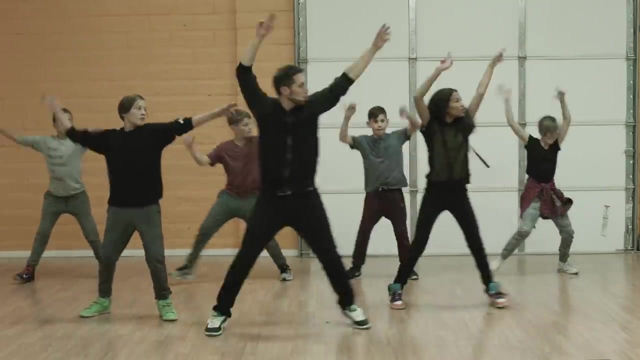 or keep it minimalized and do more footwork, dance as it goes. Okay, That completes the entire chorus, So let's do it again for them. Here we go, 5,, 6, and sing Because you are good and I dance because you are good. 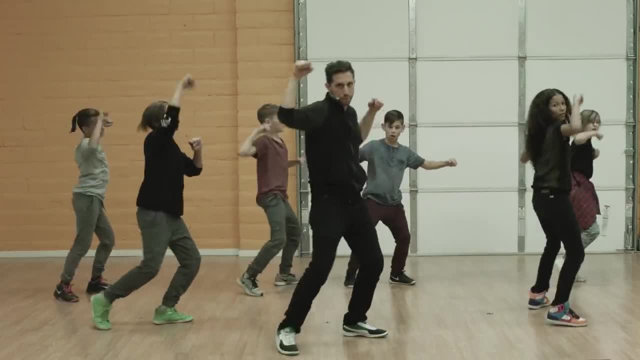 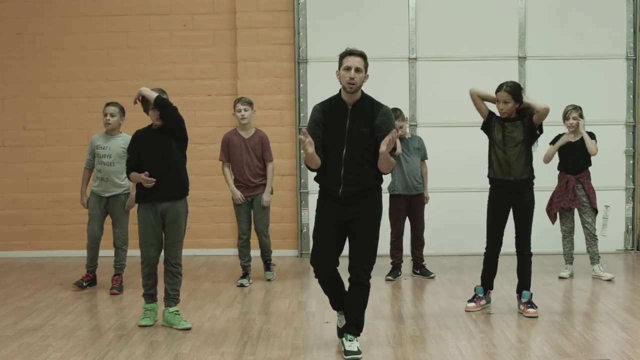 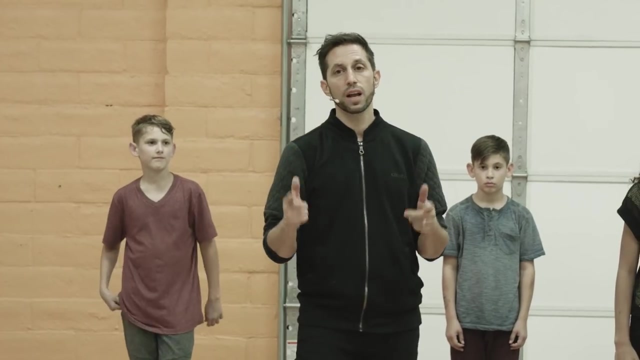 and I, because you are good to me- Boom, boom, boom. Okay, And that completes the chorus, for you are good. Next up, we're going to have the chorus with music, All right. So now we're at the point where we're going to do it with music. 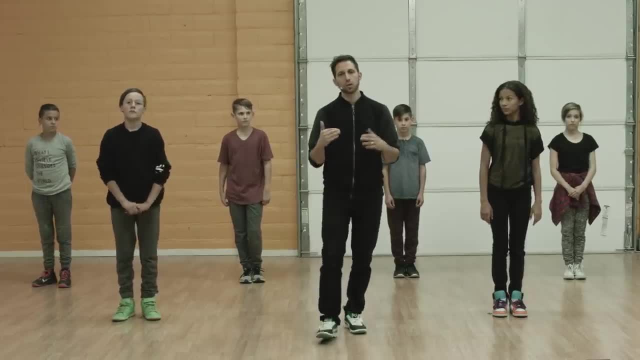 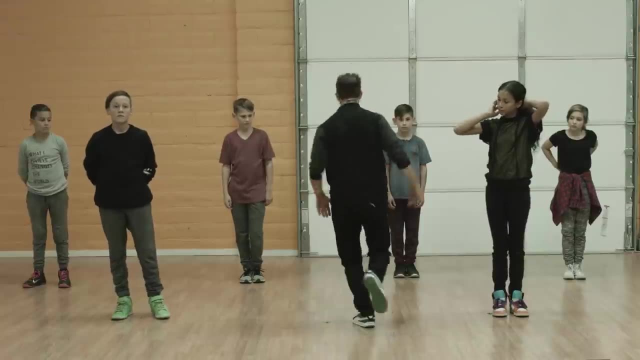 This is: you are good chorus. This is: you are good with the chorus, with the music. The chorus repeats itself twice. So once you finish the movement, 1,, 2,, 3,, 4,, 5,, 6,, 7,, 8,. 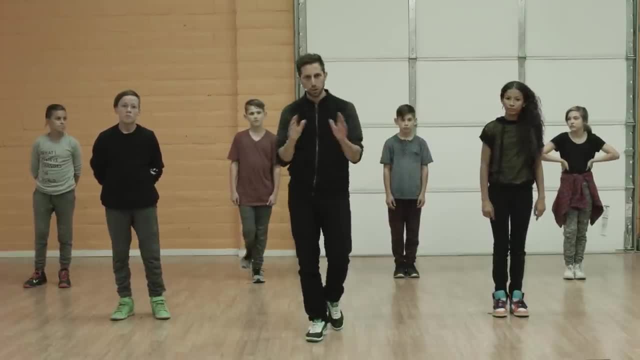 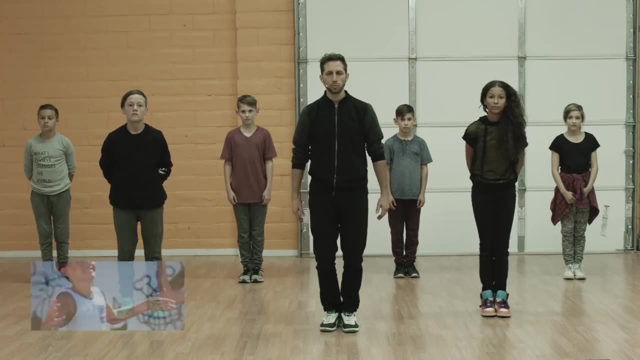 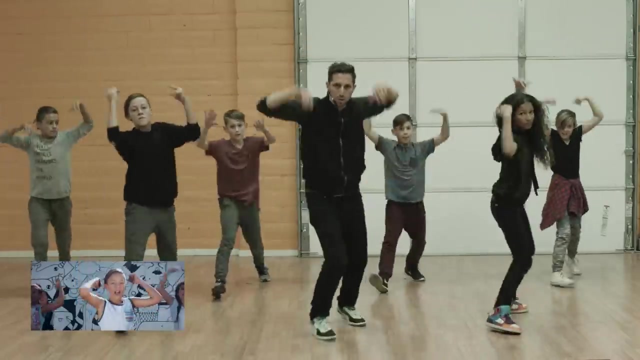 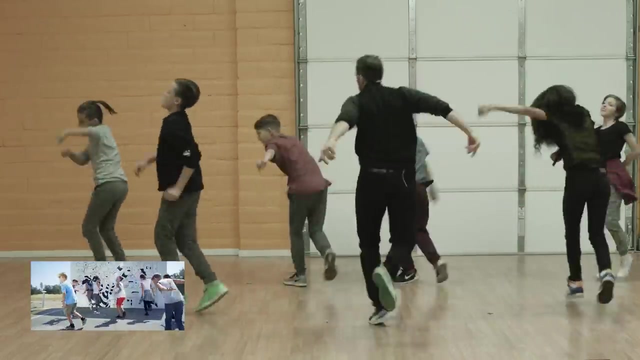 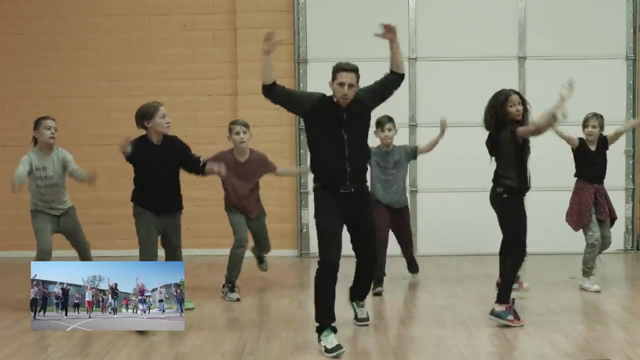 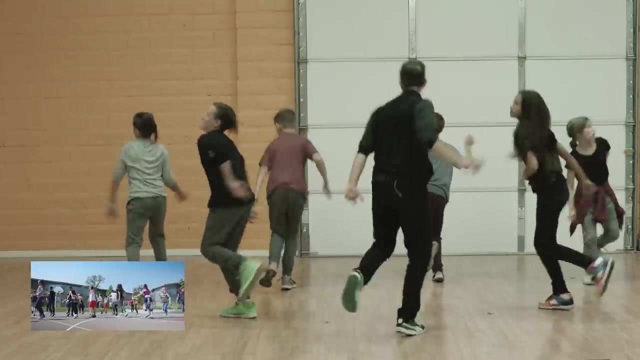 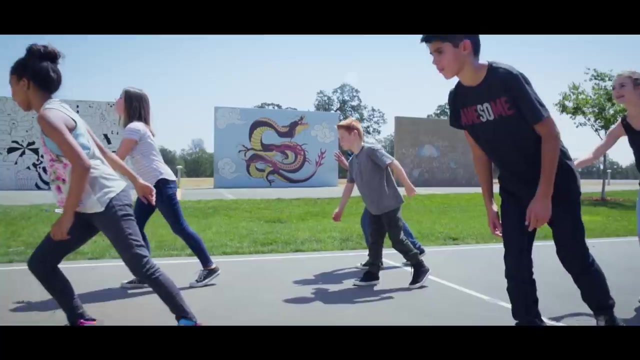 you go back into this one more time to complete the full chorus section. Okay, So here we go. You are good with music chorus. You are good, and I shout because you are good. You are good to me. Nothing and no one comes anywhere close to you. 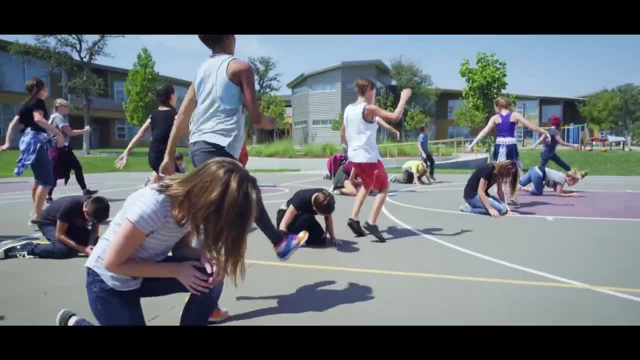 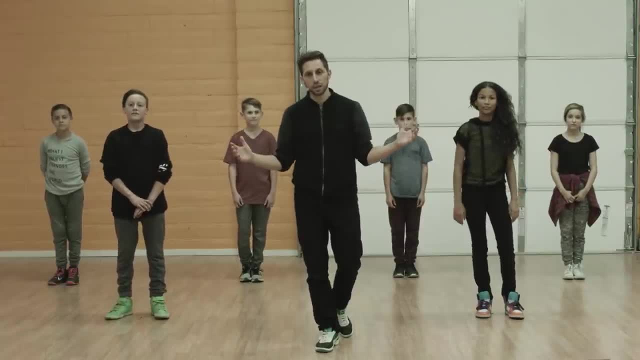 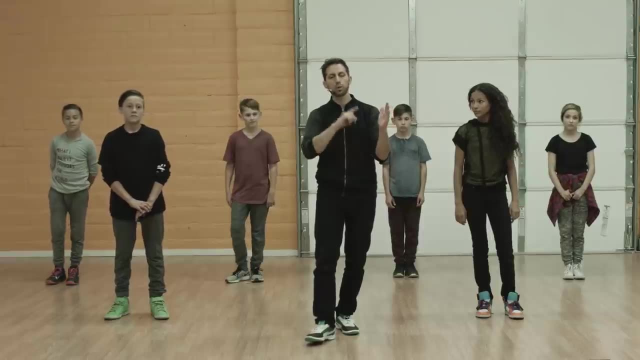 The earth and oceans deep only reflect this truth. All right, So now we're at the end of the tutorial. What we're going to be doing is going through verse 1 into the chorus with music. So we're going to put all that together with music. 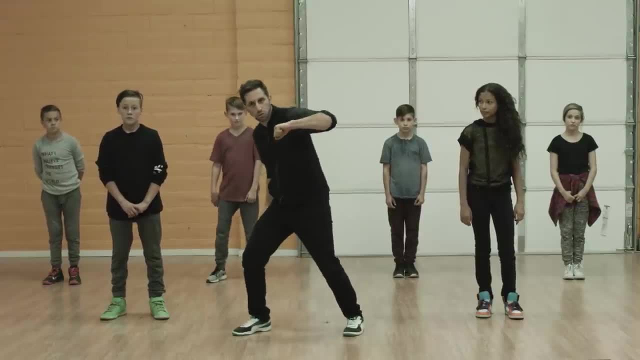 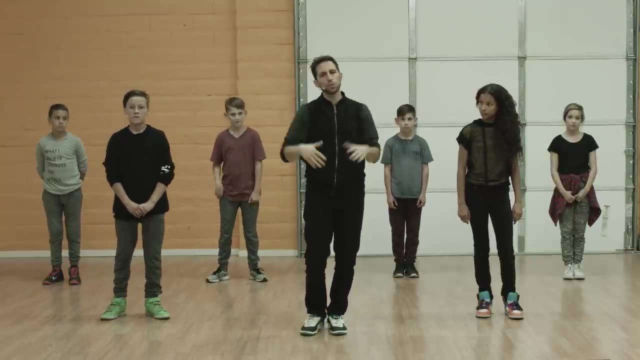 Keep in mind that right at the end, after the first verse there here you have a one eight count transition that leads into the chorus, And that's a moment for you just to freestyle, have fun with that eight counts and then go right. 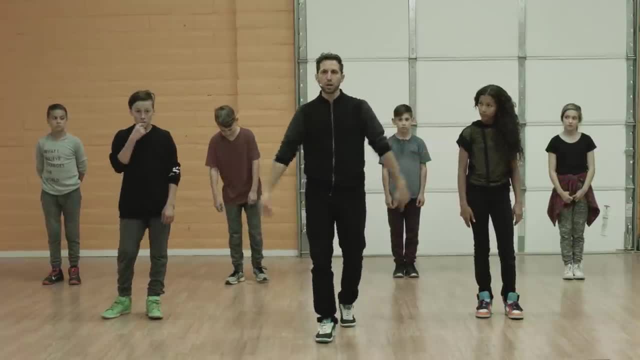 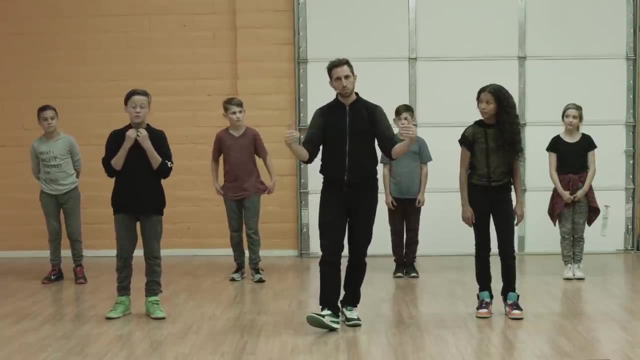 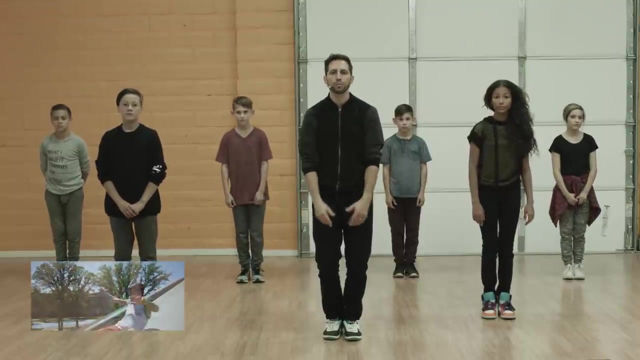 into the movement. We'll demonstrate our kind of freestyle moment, But remember dancing. this is your time to just feel the freedom that comes through movement, And so let's do it together. Ready Verse 1 and chorus 1, 2, 3, 4, 5,, 6,, 7, 8..